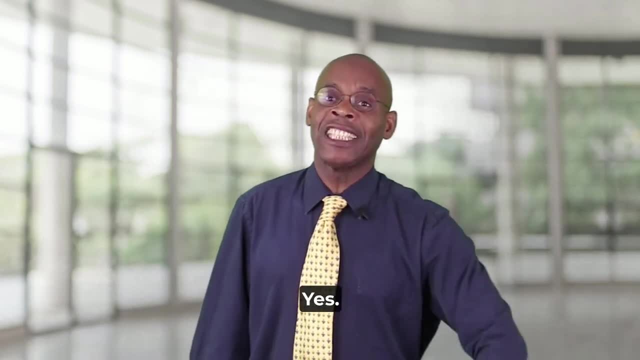 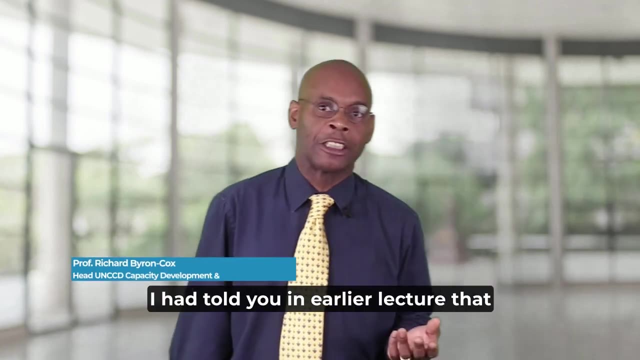 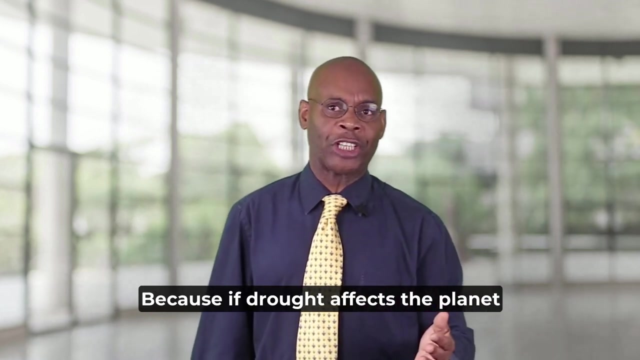 and for taking time to listen to these lectures. Yes, so today we look at various areas of the world where droughts do occur. Now, I had said in an earlier lecture that drought affects the planet generally. So then, why do we need to do this? Because if drought affects the planet generally, then we can leave it there. 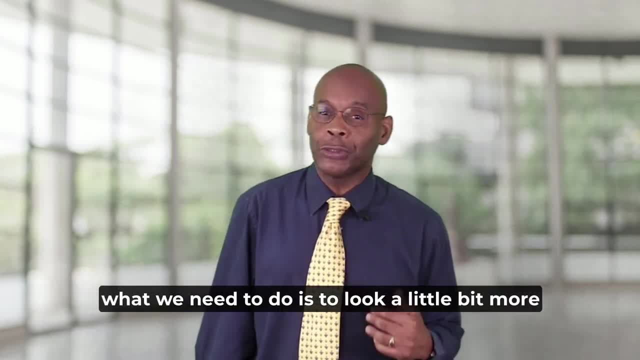 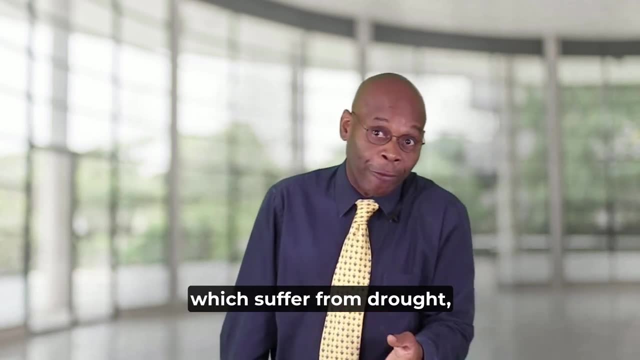 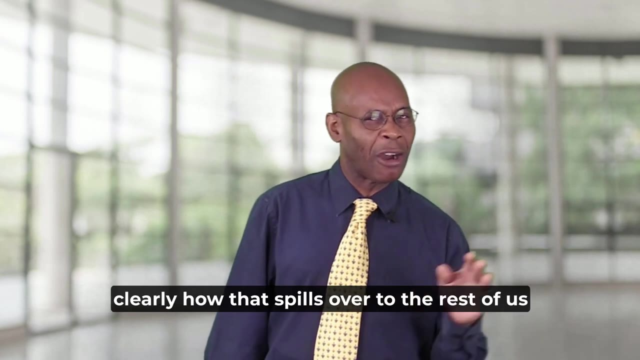 Well, not so fast. really. What we need to do is to look a little bit more carefully as to the regions of the world which suffer from drought, why they suffer from them, but also because we want to understand more clearly how that spills over to the rest of us which do not directly suffer from them. 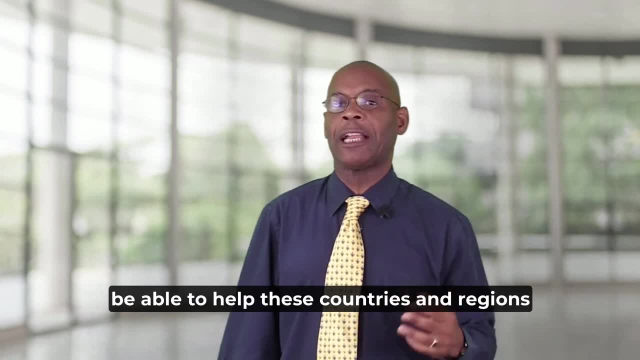 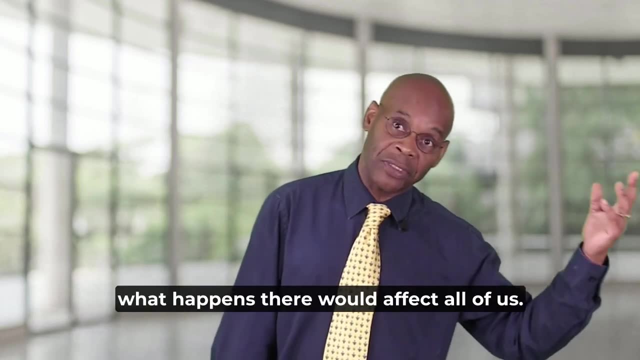 We also want to understand how we might be able to help these countries and regions, you know, in terms of dealing with drought. okay, Because ultimately, what happens there would affect all of us. So let us look at some of the areas of the world where drought occurs. 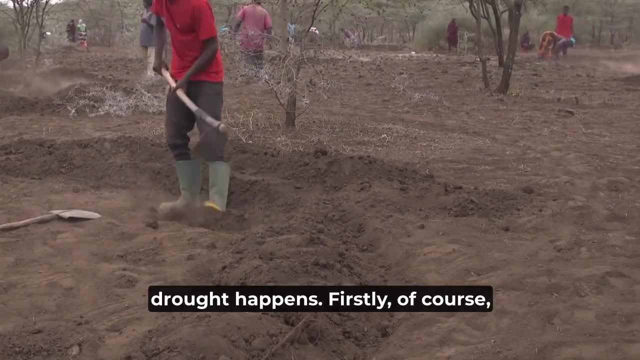 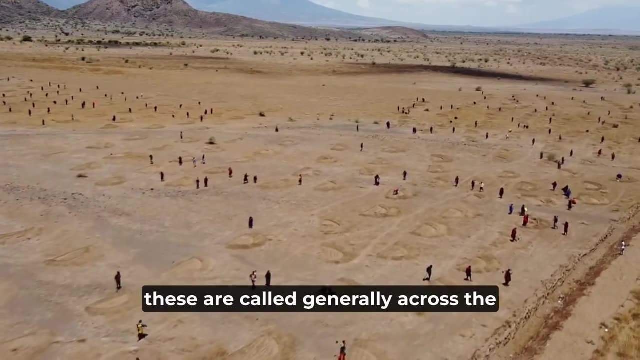 It's prevalent or where drought happens. Firstly, of course, we should look at the lands which are prone to drought, or the regions which are prone to drought- okay, Now, these are called generally across the globe, wherever they are found, and they are found all over the planet. 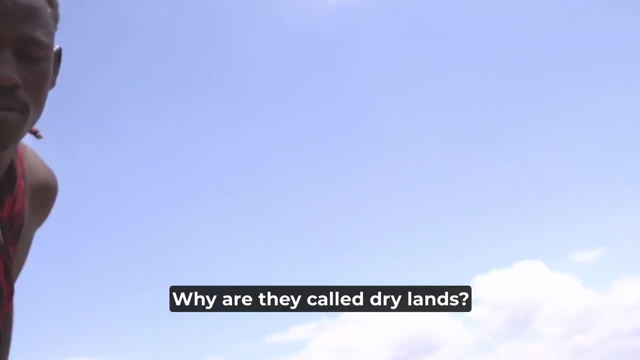 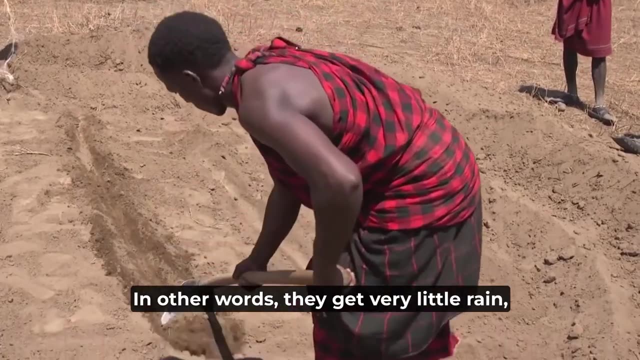 Wherever they are found, they are called dry lands. Why are they called dry lands? Well, the main reason for this is because they have what is called low precipitation, In other words, they get very little rain, very little snow or very little sleet, and this leads to what 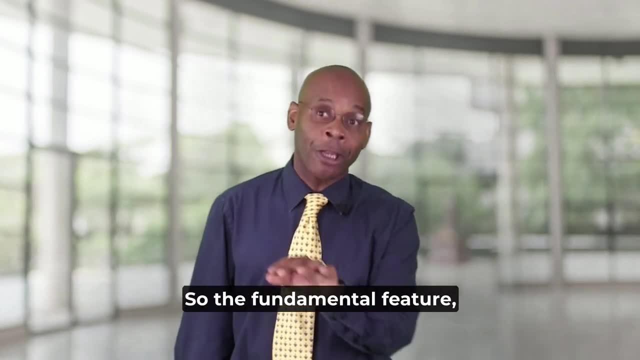 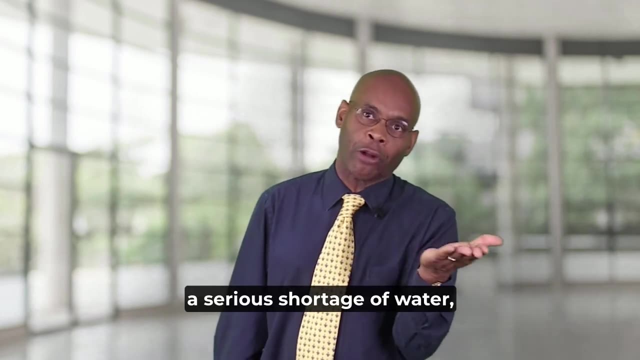 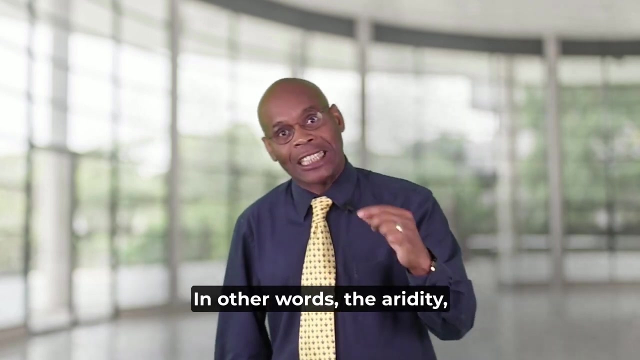 This leads to a shortage of water. So the fundamental feature, the common feature of all of these lands right is that they have a serious shortage of water right And that is why they are called dry land. In other words, the aridity, the dryness of these areas right is what pacifies them as such. 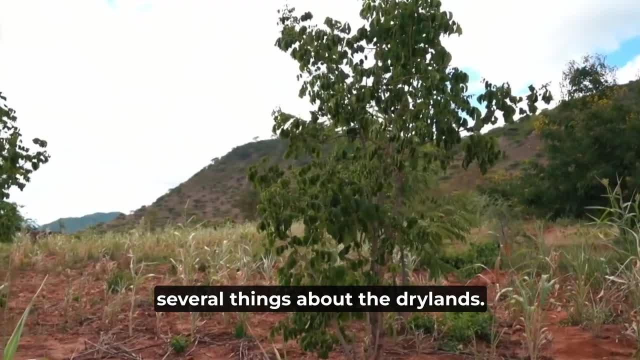 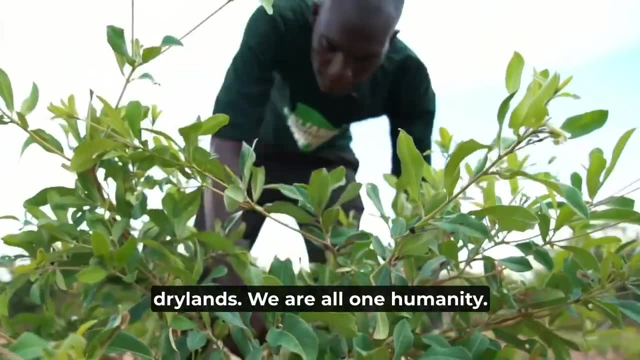 Now it is important for you to understand several things about the dry lands. In the first place, at least 2 billion people live in these dry lands. We are all one humanity. We cannot be indifferent to the fate of 2 million people when they are affected by drought. 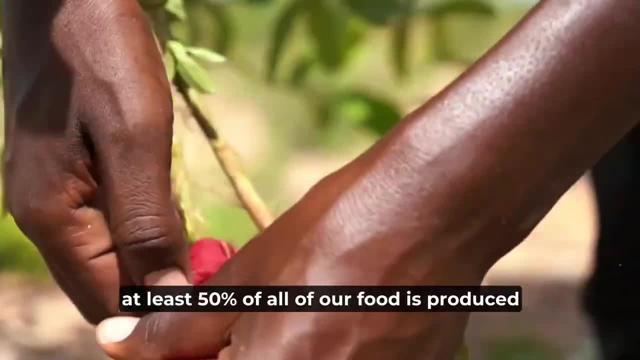 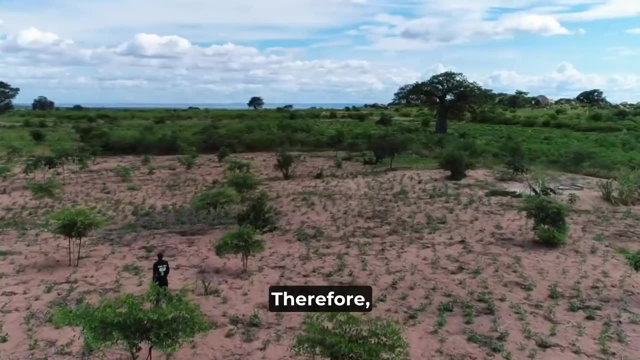 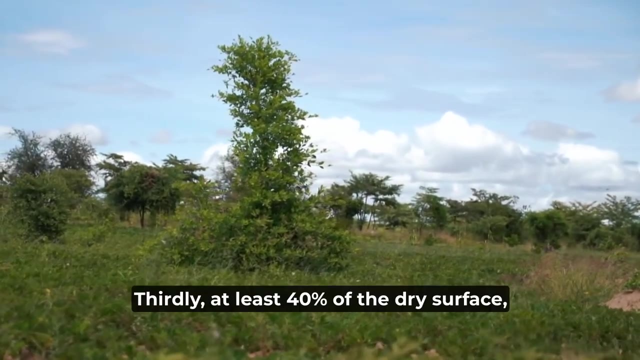 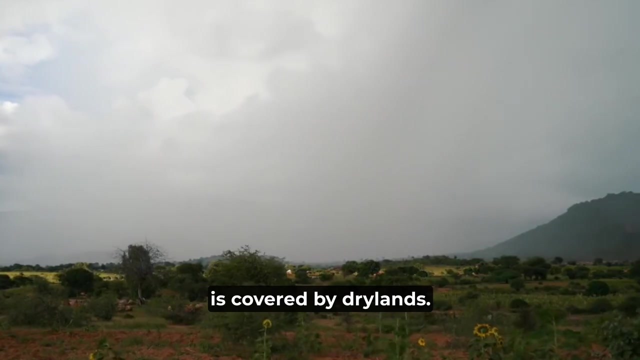 That's the first thing. Secondly, at least 50% of all of our food is produced in these dry lands. okay, Therefore, serious drought in these areas also does what Affects our food security. Thirdly, Thirdly, at least 42% of the dry surface, the land surface of our planet is covered. 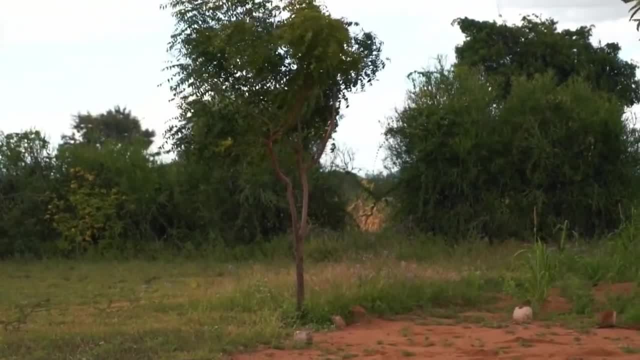 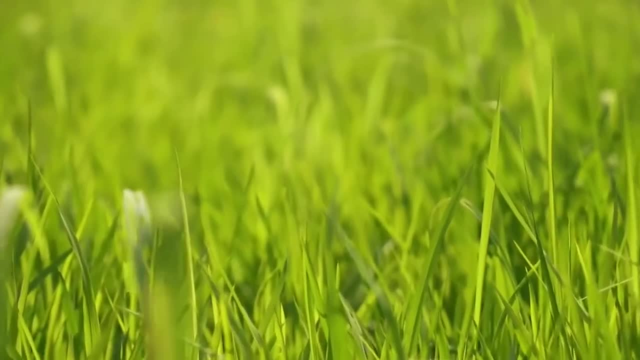 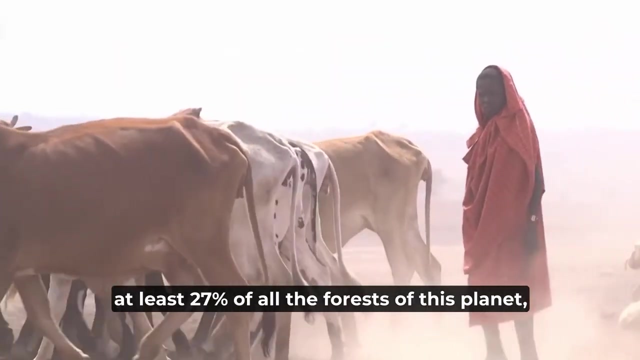 by dry lands. That's a significant portion of the global land space, So we have to be interested in that sort of stuff. Fourthly, at least 27% of all the forests of this planet, 27% of global forests, is located. 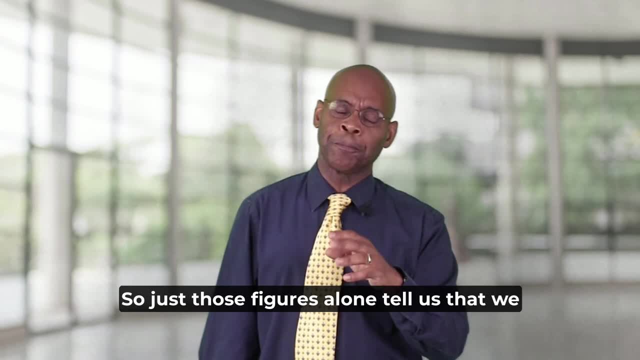 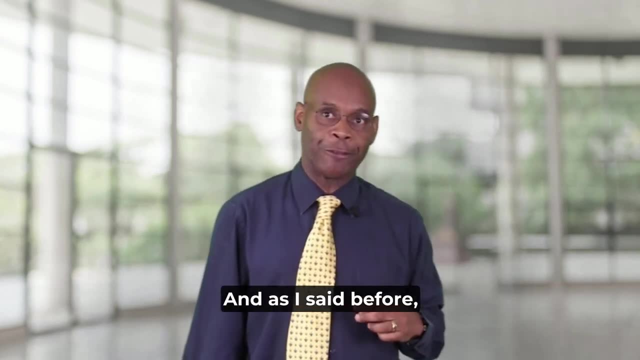 in the dry lands. So just those figures alone tell us that we need to be concerned with the dry lands, even if we don't live there. And, as I said before, dry lands can be found in Asia. they can be found in Africa. they. 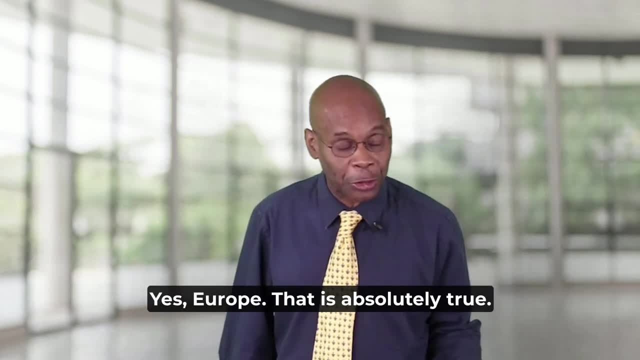 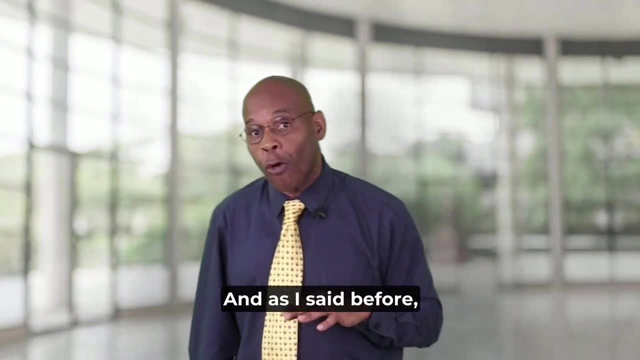 can be found in the Americas, and they can also be found in Europe, Yes, Europe, That is absolutely true. So those are the dry lands, But it's not just the dry lands and, as I said before, there was this false understanding. 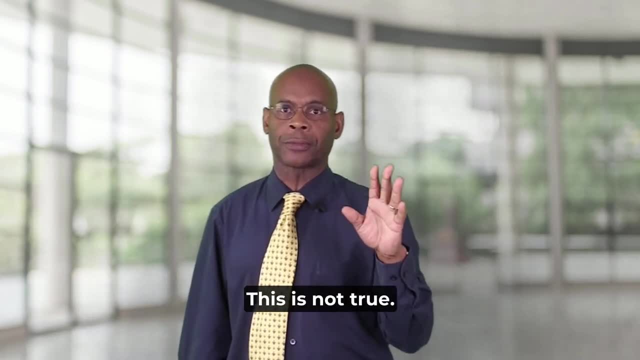 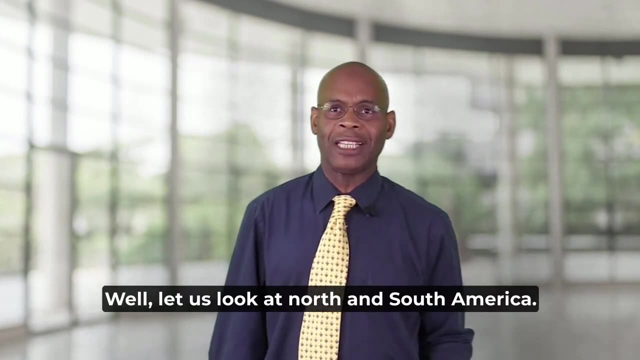 that dry land is not the only thing that can be found in the dry lands. Drought only happened in the dry lands. This is not true. Okay, let us turn to the Americas Now, and well, let us look at North and South America. 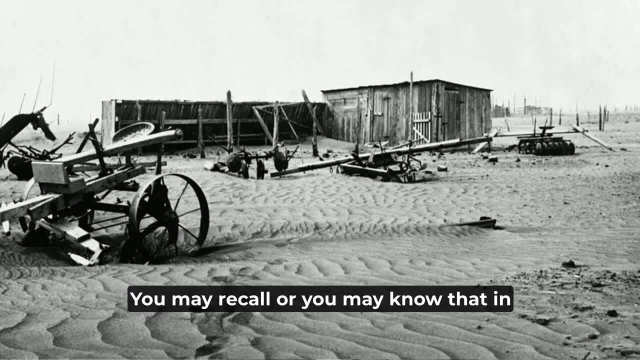 Let's begin with North America. You may recall, or you may know, that in the 1930s and 1950s there were very, very serious droughts in North America. A matter of fact, in the 1930s there was something called the Dust Bowl Phenomena. 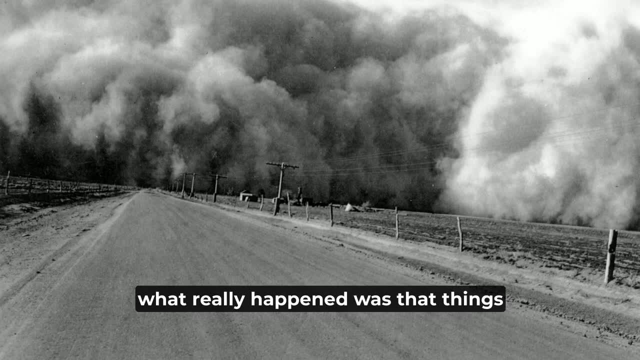 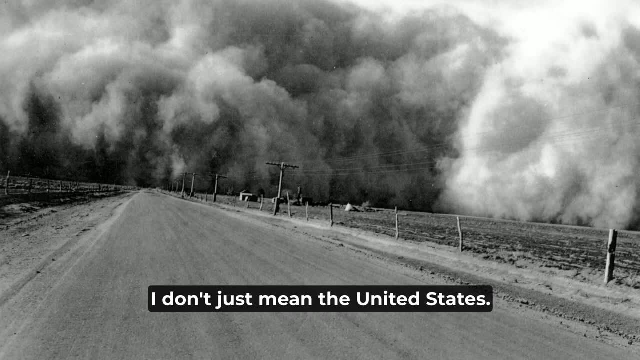 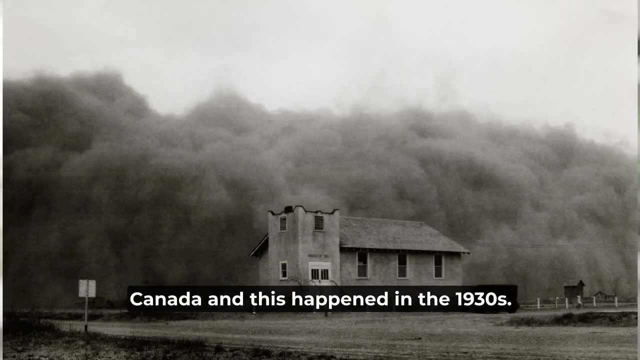 in North America, And when I say North America, I don't just mean the United States, It was more the Peary lands, meaning the lands shared by the United States and Canada. okay, And this happened in the 1930s. 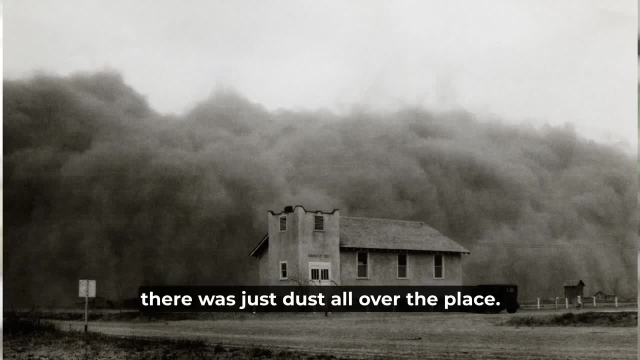 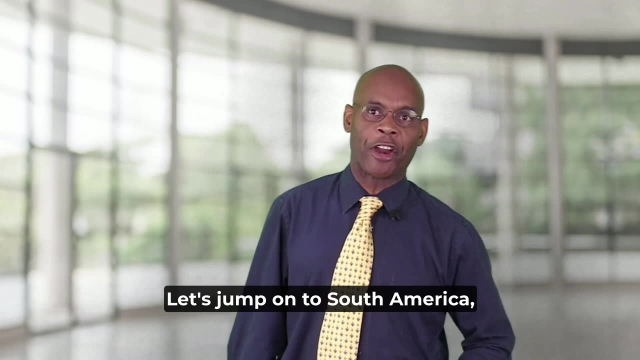 It was so bad, the place was so dry, there was just dust all over the place, you know, and that is why it was called Dust Bowl Phenomena. That is North America. Let's jump down to South America and let's deal with Brazil, which is the biggest country. 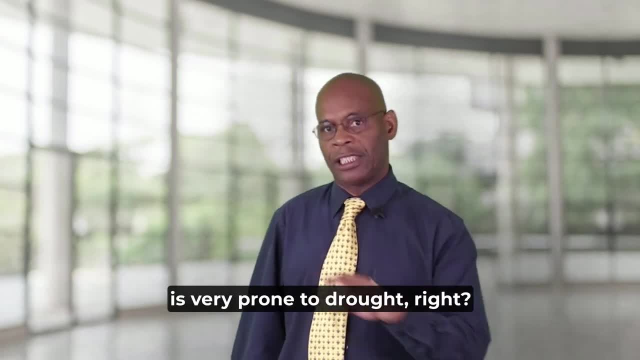 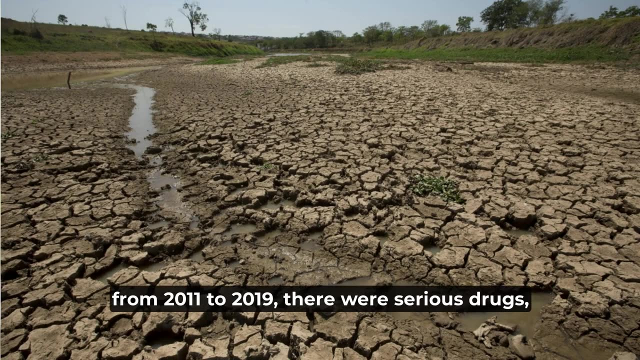 in South America. Now, the northeastern side of Brazil is very prone to drought, right A matter of fact, from 2011 to 2019, there were serious droughts right in Brazil. Further, between 2014 and 2019,, the authorities in Brazil, the government authorities in Brazil, 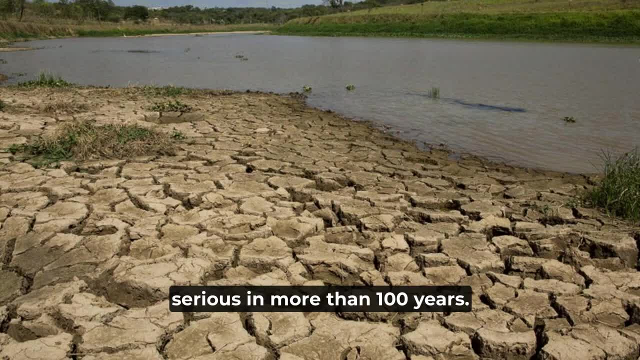 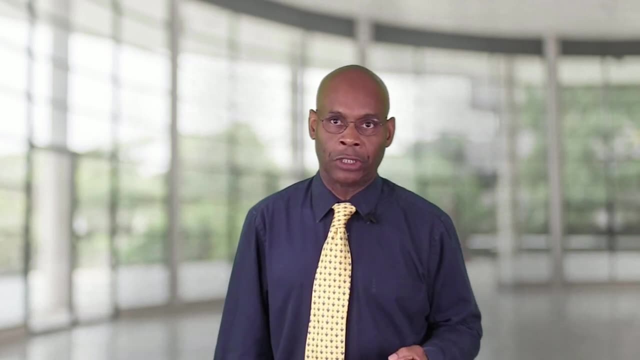 said, the droughts that took place at that time are the most serious in more than 100 years. Do you understand what we're talking about here? And this is just the Americas? you understand That drought has this really bad effect, you know, on many parts of the world? 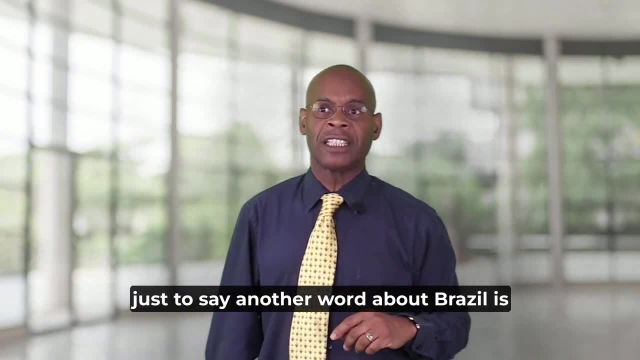 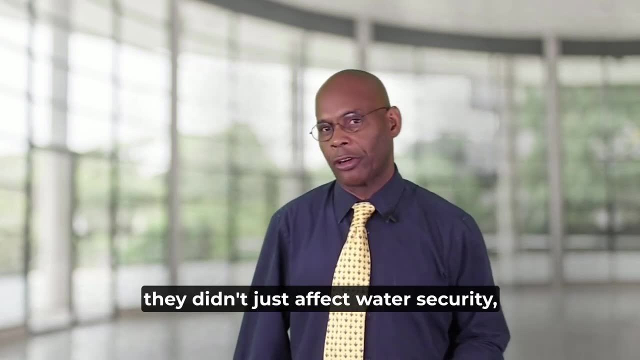 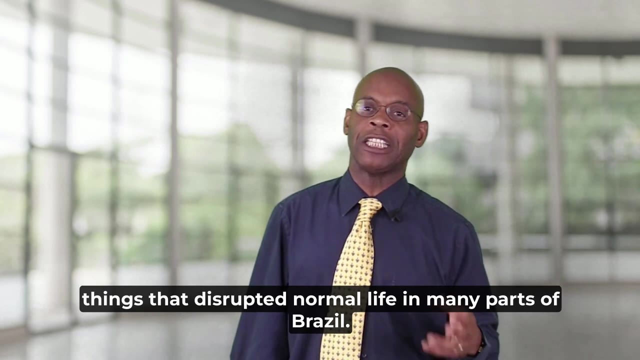 Now just to say another word about Brazil is that when those droughts occurred, they didn't just affect, They affected. They affected water security, They affected food security and many other things that disrupted normal life in many parts of Brazil. We must understand that. 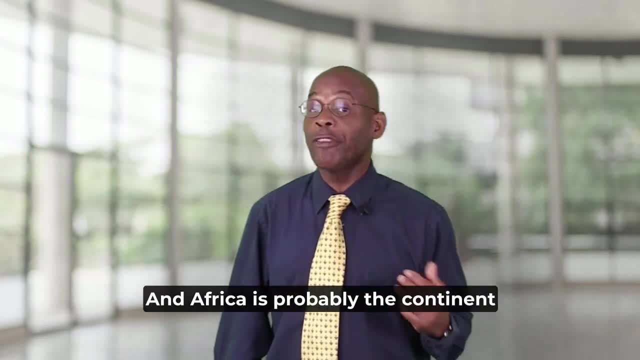 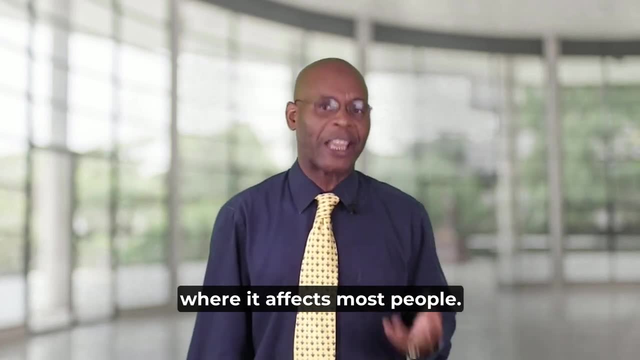 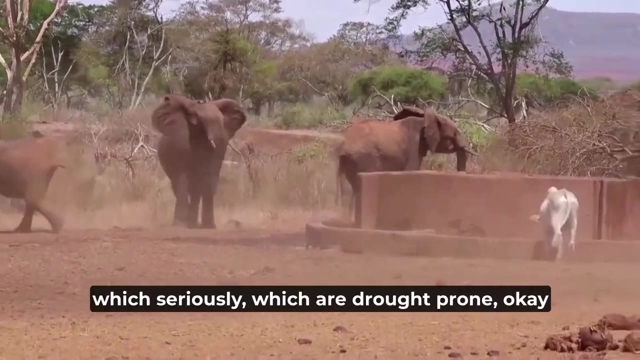 Now let's go to Africa, And Africa is probably the continent where drought is most severe, where it affects most people. As we know, there are two regions in Africa- the Sahel and the Horn of Africa- with seriously which are drought-prone. okay, 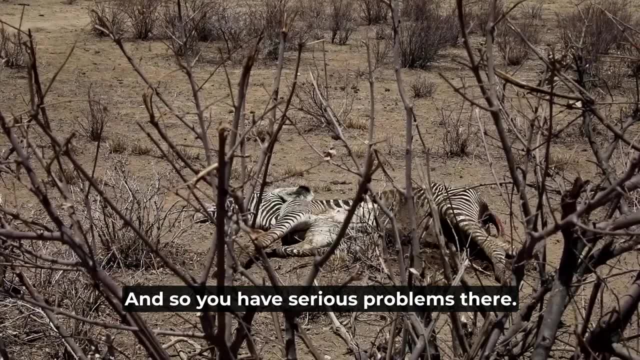 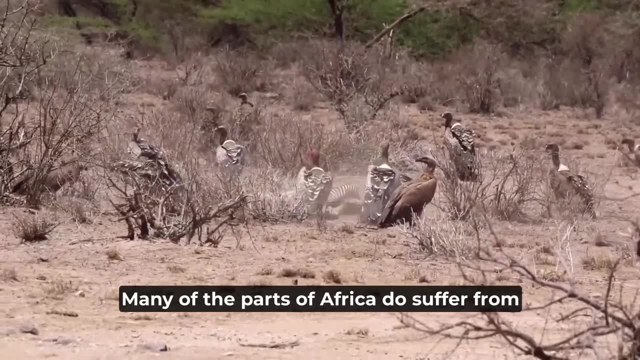 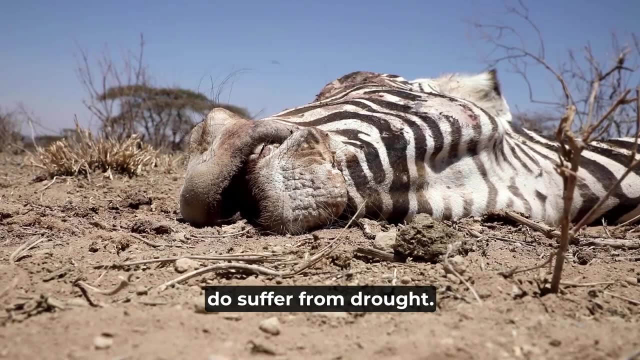 These are dry land areas And so you have serious problems there. But it's not just the dry land areas of Africa, right? Many of the parts of Africa do suffer from drought, from the south right up to the Maghreb region do suffer from drought.